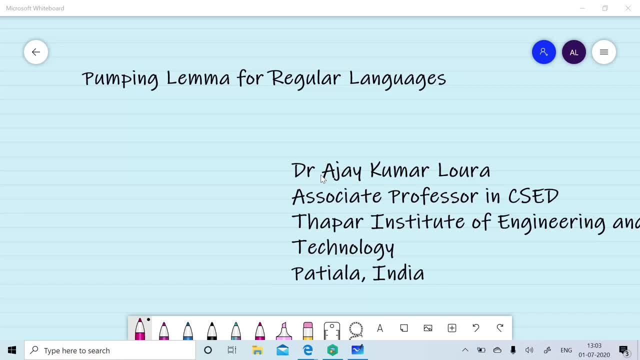 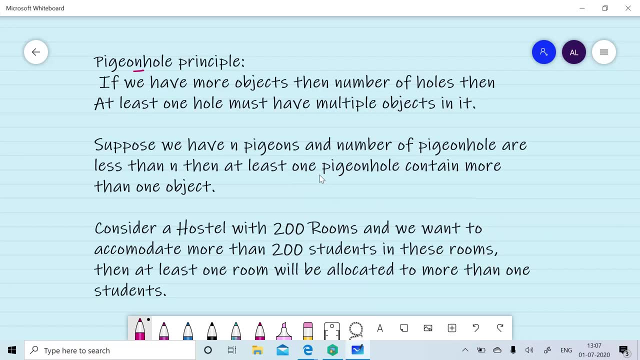 Pumping lemma is not used to prove that certain languages are regular one. Let's start the session. Pumping lemma is based on pigeonhole principle, So first we will discuss what is the meaning of pigeonhole. If we have more objects than the number of holes, then at least one hole must have multiple. 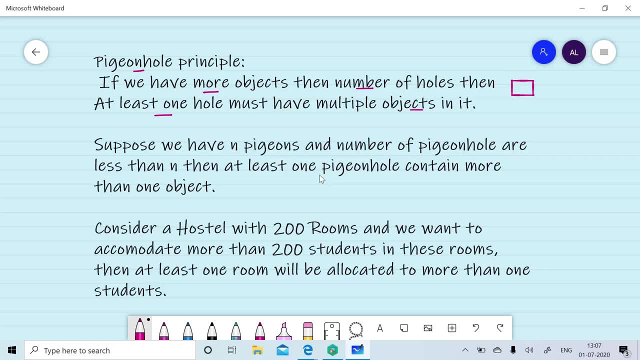 objects in it. Consider: we have three holes and we want to accommodate five objects in these ones. If we will put first object in the first one, second in the second one and third in the third one, we are left with two objects. They will be occupied in either one. 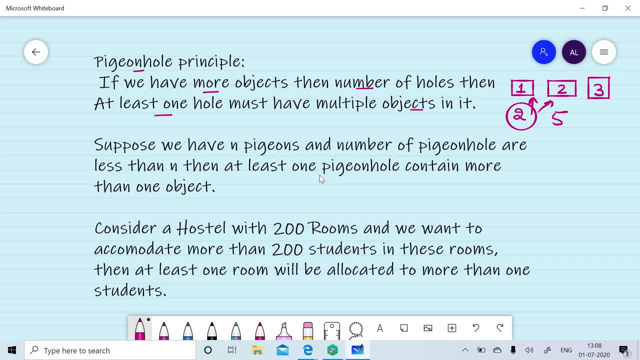 of these. So at least one pigeonhole must have multiple objects in it. Consider: we have n pigeons and number of pigeonholes are less than n. So at least one pigeonhole contain more than one pigeons. This scenario can be considered as a hostile scenario where we have two hundred. 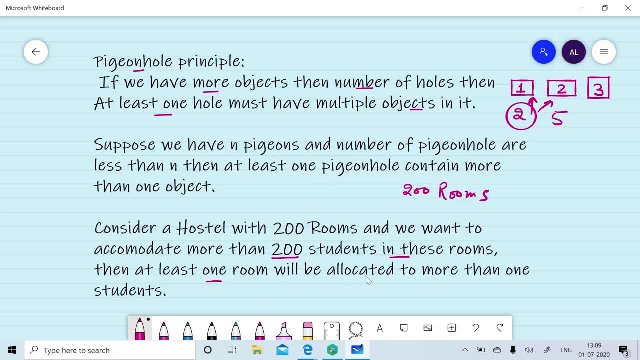 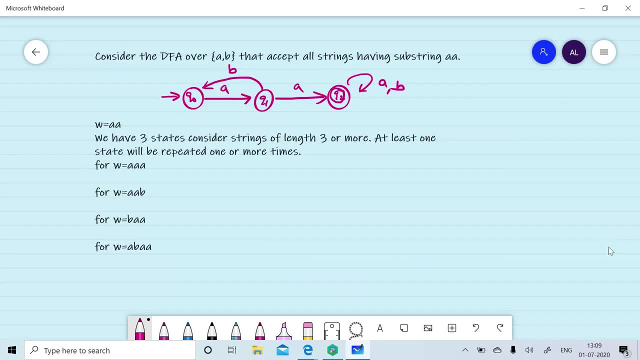 rooms and we want to accommodate more than two hundred students in these rooms, So at least one room will be allocated to more than one student. dfa that accept all string having substring aa. so number of states are 3. minimum string for which we can able to move from q0 to qf is of length 2 w, equal to aa on q0. if we will read a. 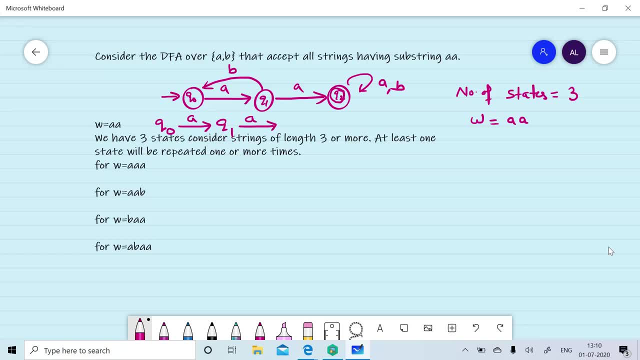 we will move to q1. if we will read a on q1, we will move to qf. now, if we have three states and we will consider string of length three or more, then at least one state will be repeated one or more times. for example, if you will consider the string aaa on q0, if you will read a, 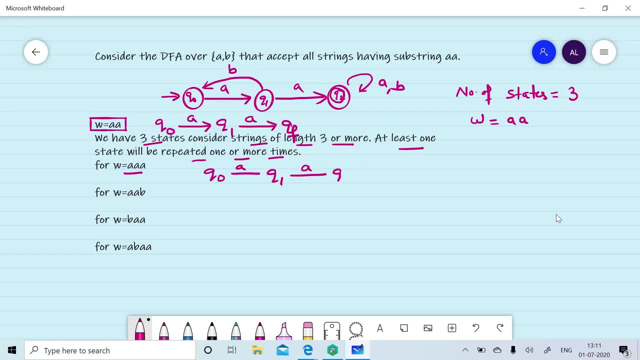 we will move to q1. if you will read a on q1, we will move to q2 again. if we will read a, we will move to q2. so here q2 state is repeated two times and the length of w is three. say similarly: if we will take w is aab on q0. if we will read a, we will move to q1 again. if we will. 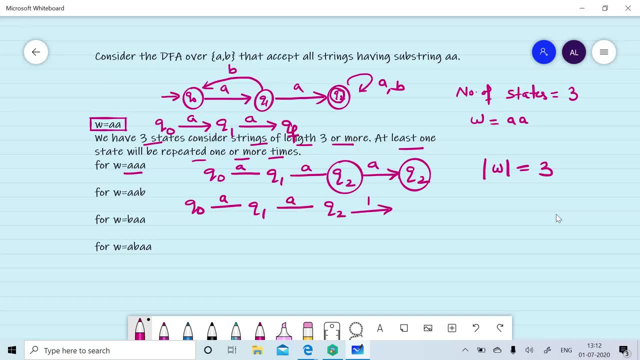 read a, we will move to q2 again. we will read b. we will move to q2 again. q2 is repeated two times if we will take baa. so if we will read b on q0, we will remain in q0. if we will read a, we will. 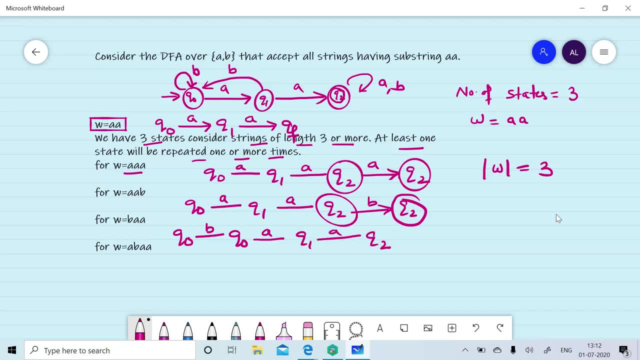 move to q1, we will read a. we will move to q2. here q0 is repeated two times and the length of w is again three. if we will take w is of length four, a, b, a, a. if we will read a on q0, we will move to q1. if we will read b, we will come back to q0 again. if we 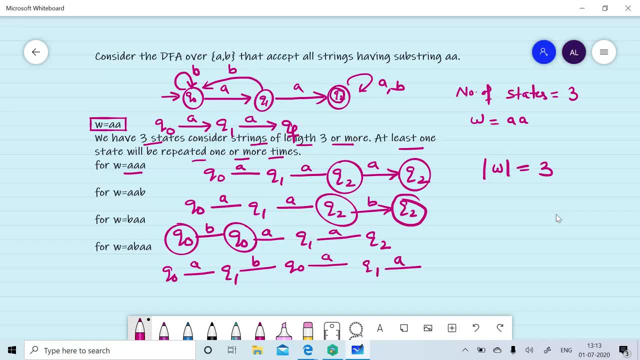 will read a, we will move to q1 again. if we will read a, we will move to q2. here q0 is repeated two times. q1 is also repeated two times. so in general, if we have a dfa with three states and if we will take any string w that belongs to the language and its length is greater than equal, 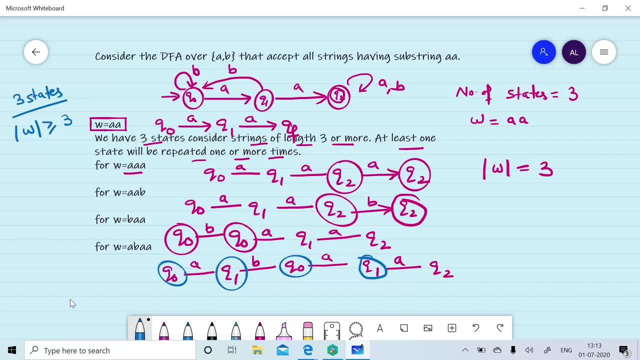 to three, then at least one state will be repeated one or more times. we can generalize it if: if there is n states in our dfa and if we will take a string w with the length greater than or equal to n, then there exists at least one state that will be repeated one or more times. now we will discuss. 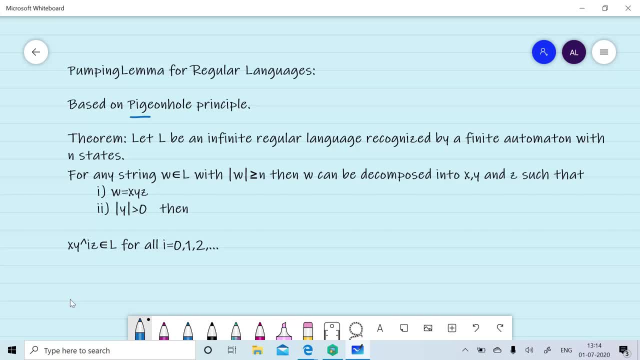 pumping lemma for regular languages. now we will discuss pumping lemma for regular languages first is it is based on piezel whole principle. it can be described by this theorem: let l be an infinite regular languages recognized by a finite automata with n states. then if you will consider 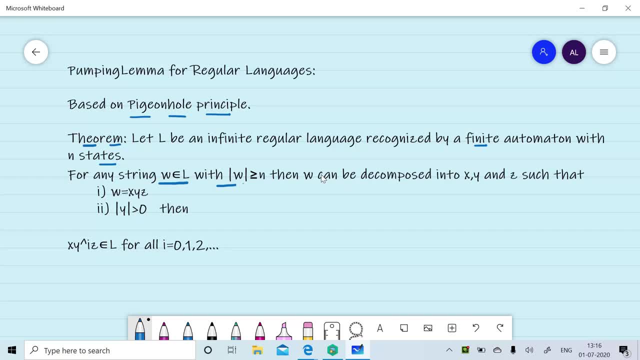 any string w belongs to the language with, with the condition that the length of w is greater than equal to n, as we had discussed previously, then w can be divided into three parts. we can able to divide w into x y z, and then we can divide w into x y z, and then we can divide w into x y z. 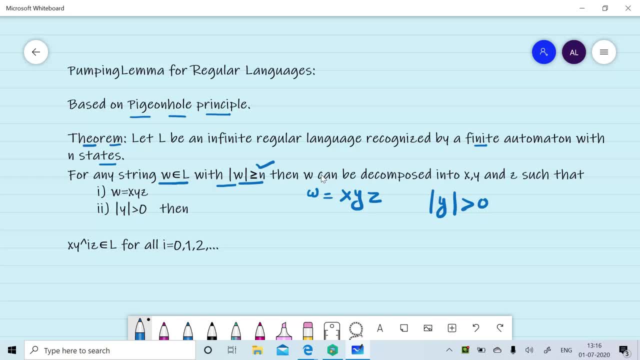 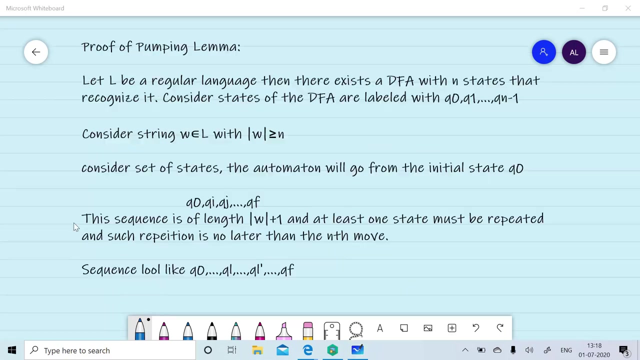 length of y is at least one, then x, y, key power i, z will belongs to the language, for i is greater than equal to zero. what it means: x- z belongs to the language, x, y z will belongs to the language. x y square z will belongs to the language, and so on. now we will discuss the proof of pumping lemma. 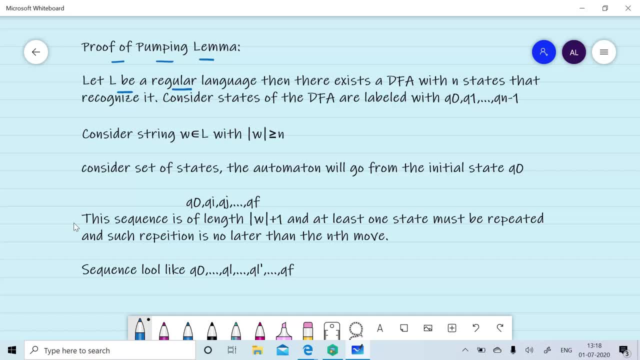 let l be any regular language so we can able to design a dfe with n states. we can call this n state as q0, q1, qn minus one, and if we will take any string, w, with, with the condition that length of w is greater than equal, 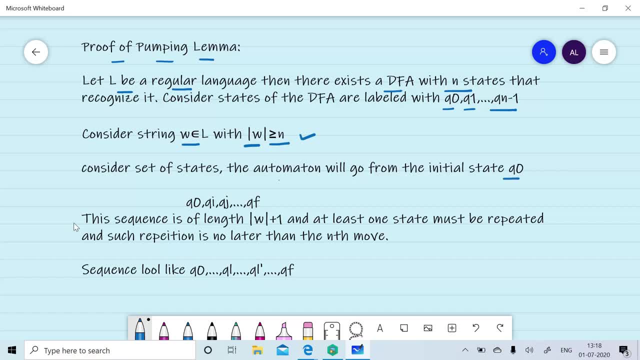 to n. then the automata will go from the initial state q0 to qf. initially it is in q0, let's consider: then it will move to ky, then it, then it is moving to kj, and so on. in the last it will reach to qf state. 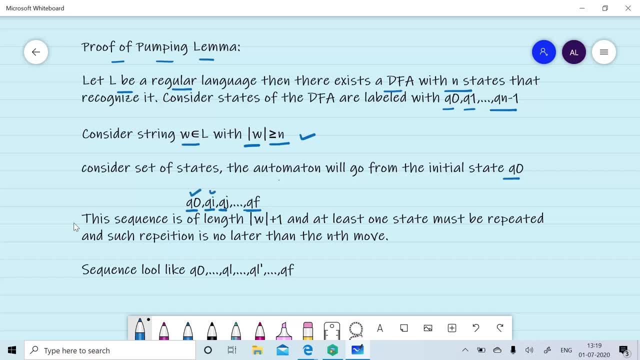 so this sequence, q0, qi, qj up to qf, is of length w plus one, because initially we are in q0. after reading each symbol we are moving to a new state. so length of w plus one is the number of states that we had visited, and at least one state will be repeated, because the number of states are n. 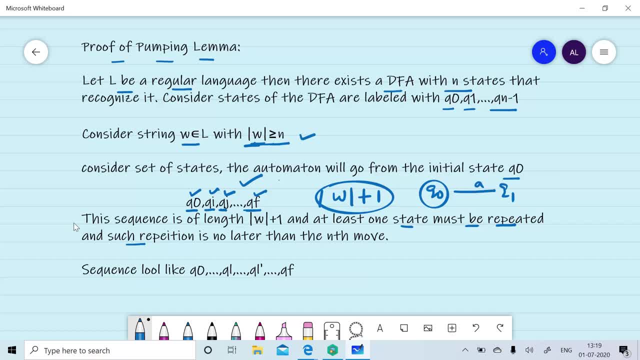 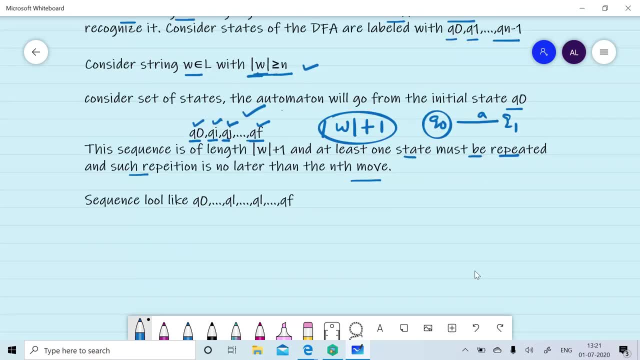 and we had considered the string of length greater than equal to n, and such repetition is no later than nth move. so we can say that at least one state will be repeated. let's call it as ql state. so we will start with q0 after reading a number of symbol. 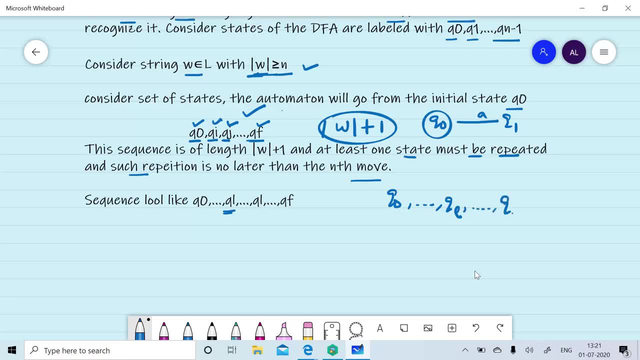 we will move to ql. then, after reading a number of symbol, we will again move to ql. then, processing the remaining string, we will reach to qf. so ql state is repeated two times: pause. we can able to describe it by extended transition function, that is on state q0, if we will read string. 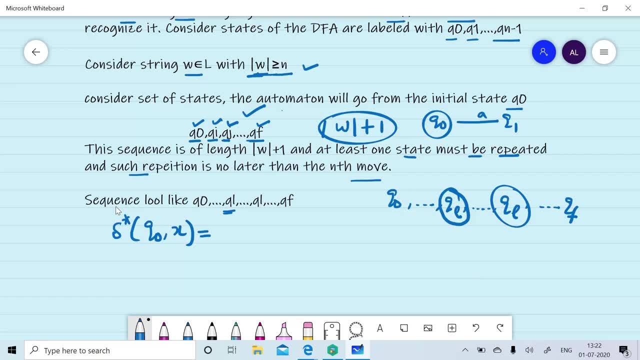 x. after processing the string x, let's suppose we will reach to ql, then from ql, after reading the string y, we will again come back to ql. so, on processing of string x, we will reach from q0 to ql. on processing of this y state, We will start from KOL and we will again reach to KOL. then, reading Z, we will move from. 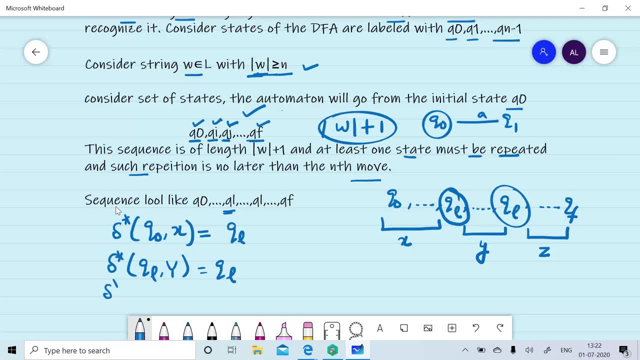 KOL to KOF. So it can be described by extended transition function, KOL Z, and we will reach to KOF with the condition length of XY is less than equal to N and length of Y is greater than equal to 1.. 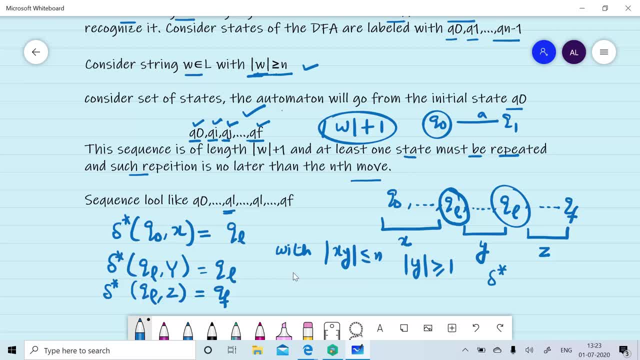 We can easily able to observe that extended transition function from KO0 to XZ will also reach to the final state. Similarly, extended transition function KO0, XYZ will also reach to the final state. Similarly, we can repeat this thing, Y, two times and we will reach into the final state. 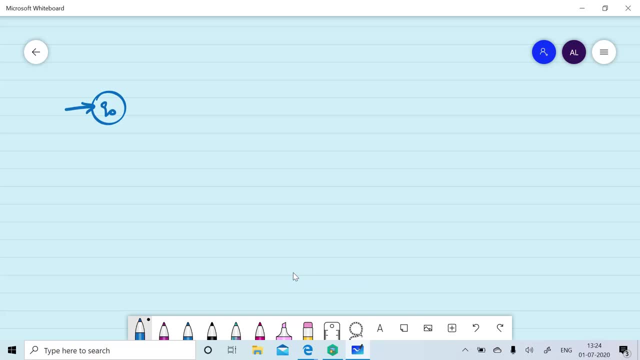 We can able to observe that extended transition function from KO0 to XZ will also reach to the final state. We can able to describe it as: from KO0 state on processing string X, we will reach to the state KOL. There may be a number of intermediate states. 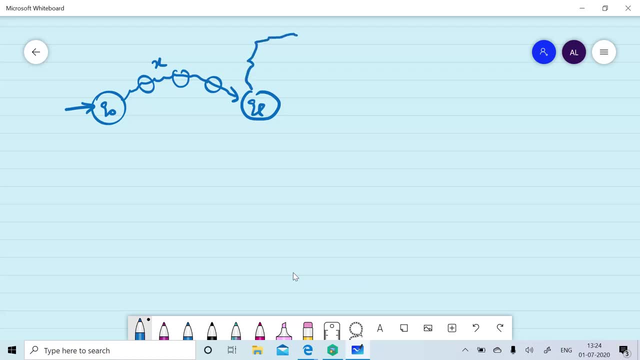 Then, on processing of Y from KOL, after reading the string Y we will come back to KOL Again. there can be a number of intermediate state. Then, on processing of Z, we will reach to the KOF state. Clearly, XZ will belongs to the language. 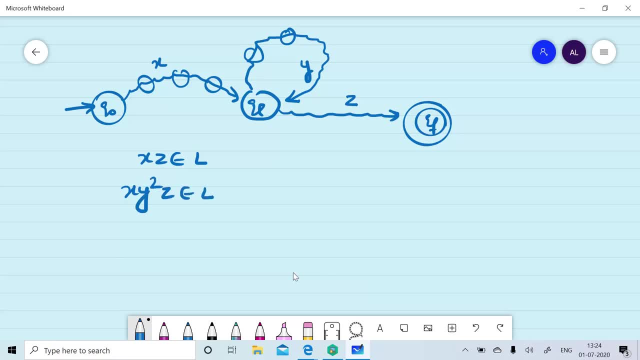 XYZ will belongs to the language, XYZ will belongs to the language, and so on. We can say that XY, key power, IZ, will belongs to L, for I is 0,, 1,, 2, and so on. Y can be pumped 0 or more times. 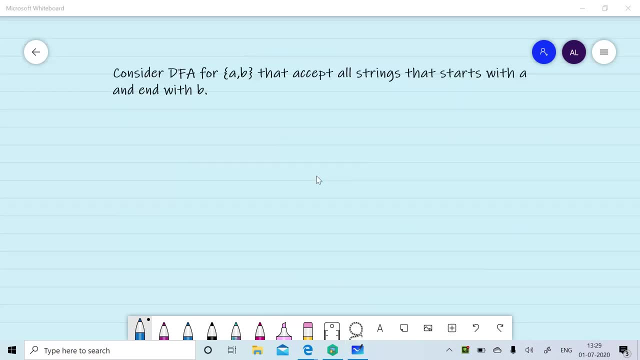 So Y can be pumped 0 or more times. So Y can be pumped 0 or more times. Now we will discuss how we can able to divide W into XY and Z. Consider an example of a DFA that accept all string that starts with A and end with B. 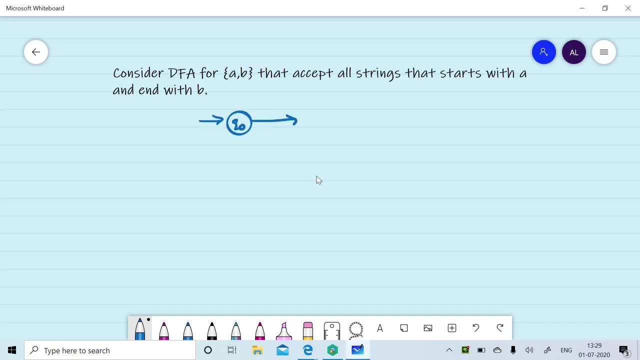 KO0, A. We are not considering the concept of rejected state over here, Because for any string belongs to the W, the rejected state will not be there. So we are not considering the concept of rejected state over here, because for any string belongs. 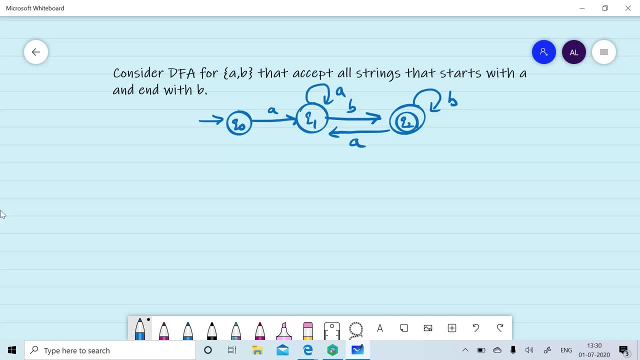 to the W KO0, A. The rejected state will not be visited. Number of states are 3.. Now consider any string WO with length greater than equal to 3.. Let's suppose we will take WO as AAB. 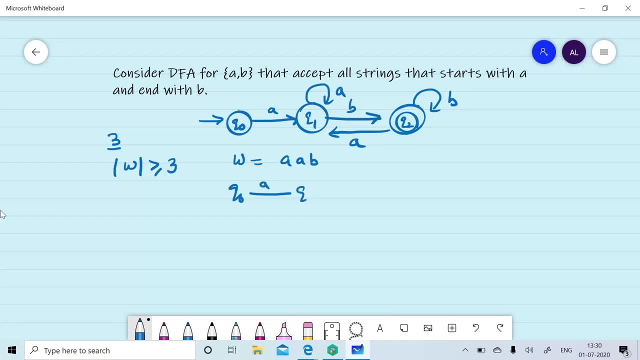 So, on KO0, if we will read A, we will reach to KO1.. Again, if we will read A, we will remain on KO1.. Then we will read B, we will reach to KO2.. Now here KO1 is visiting two times. 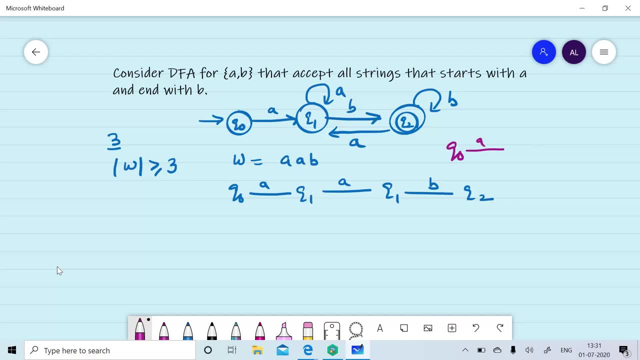 times. so we can say q0 on reading of a, we will move to q1 and then, on processing this thing, a, we will come back to a, then we will read z, that is b and we will reach to q2. so x is over, here is a. 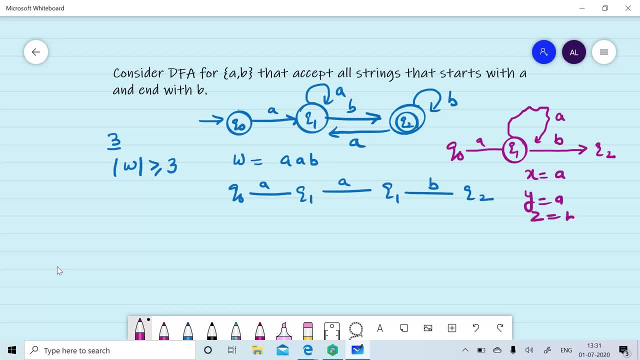 y is a and z is b. so if you can observe xz, xz is ab belongs to the language, x, y square z. that is a, a, a, b belongs to the language, and so on. now, if you will consider the string w, a, b, a, b, we will start with q0, we can read a and we will move to q1, then we will read b. 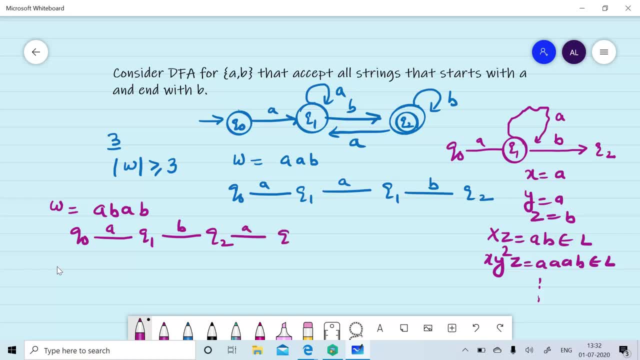 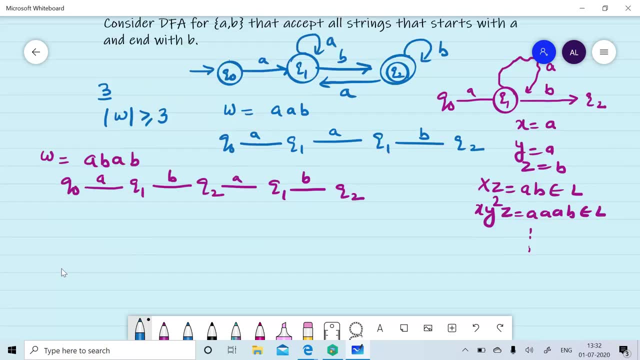 we can move to q2, we will read a. we can move to q1, then we will read b. we can move to q2. now here, q1 is visited two times. q2 is visited two times. you can consider any one of these, suppose first we will consider q1 as the state that is visited two times. we will try to find. 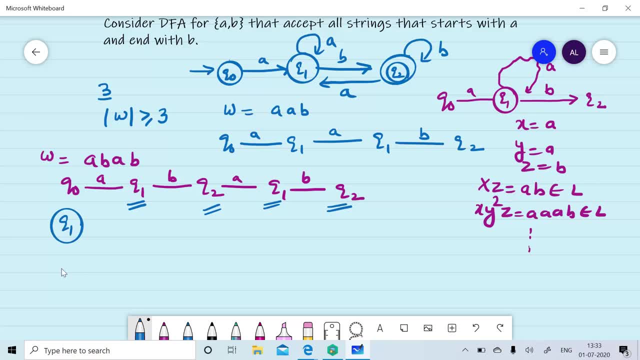 out the value of x, y and z. if, if we will consider, q1 is visited two times, so we can say q0 on reading of a, we will move to q1. then, on reading of b, and then reading of a, we will come back to q1. then, reading of b, we will move to q2. so here x is a, y is b, a and z is. 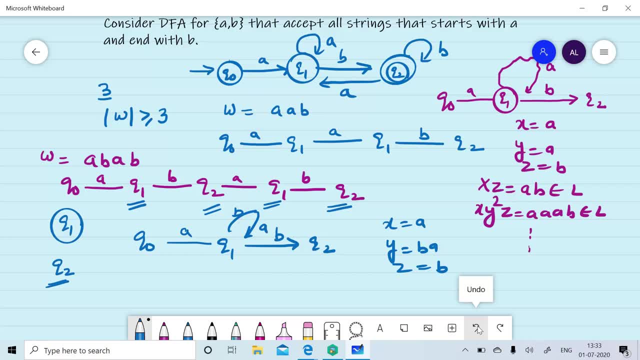 b. suppose we will consider q2 is visited two times, then q0 to a, q1 to b, we will move to q2, then on reading of a and b we will come back to q1, then reading of b, we will move to q2, then reading of b, then reading of a. but if we will observe what is the length, 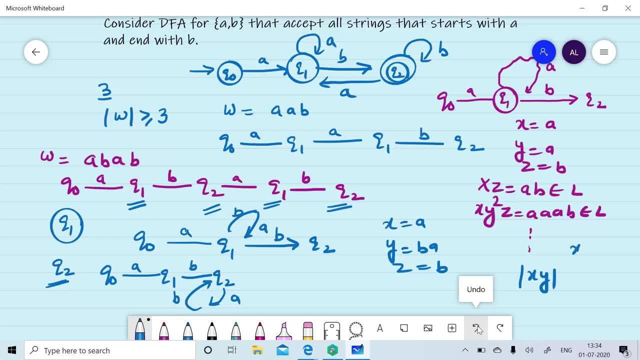 of x- y. So the length of a and b is the answer given for the length of x and y. Here x is a, b. why is ab? because from q2 we will start reading a, then on reading b we will come back to q2. so length of x- y here will become four, and that is greater than the number of state. 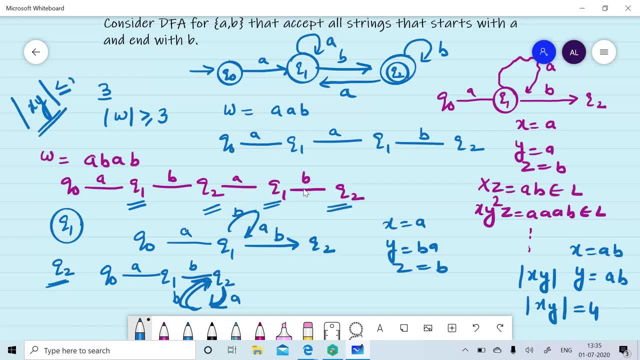 it is not following the condition that the length of x, y is 4.. Now you can implement a step or other function on thisId, and n and n is the equal to n, x, y is less than equal to n. so we cannot able to consider x, y, z as x is a b and y is a b. 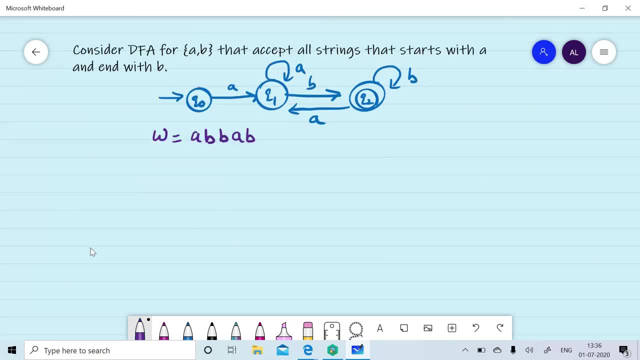 now consider w as a, b, b a b. so if we will process it- q 0 on reading of a. we will move to q 1 on reading of b. we will move to q 2 on reading of b. we will remain in q 2 on reading of a. we will. 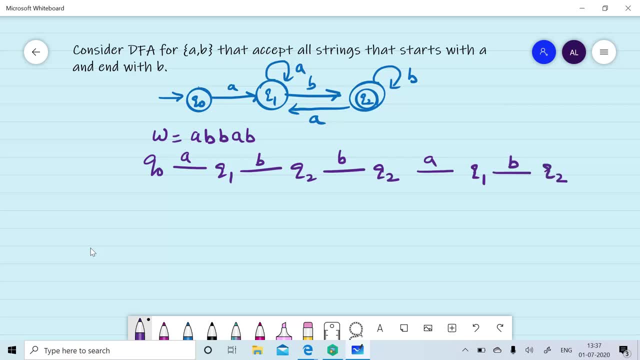 move to q 1. on reading of b. we will move to q 2. here q 2 is repeated three times, q 1 is repeated two times. so let's suppose we will consider q 2 as the repeated state. on processing of string a b. 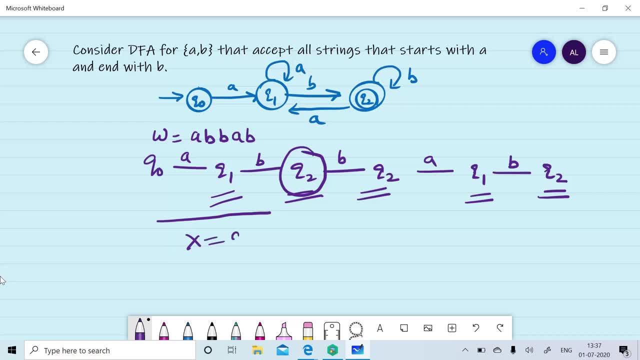 we will move from q 0 to q 2. so x is a b over here the second time it is coming, so it can be considered as. on q 0. on reading of a b string: we will move to q 1. on reading of b: we will move to. 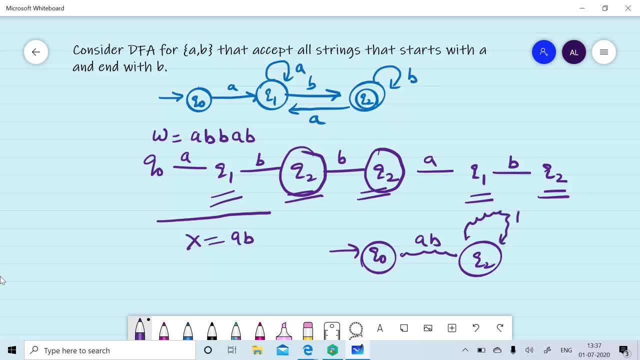 q 2. then, upon processing this string b, we will remain in q 2. then on processing of a b, we will remain in q 2. so here we can consider x as a b, y as b and z as a- b, and the length of x, y is less. 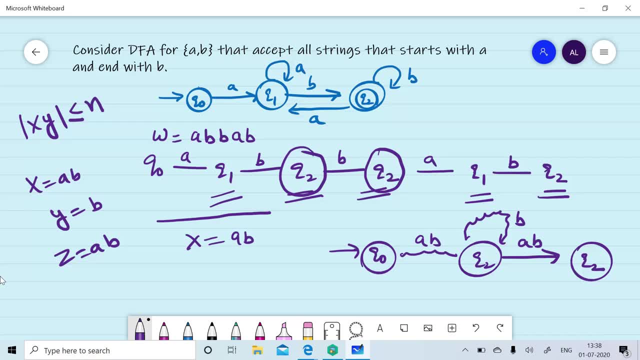 than equal to n is satisfied because the length of x- y is 3 and the number of states are 3, so we can able to consider x as a b and z as a b and z as a b, and the length of x- y is less than equal to. 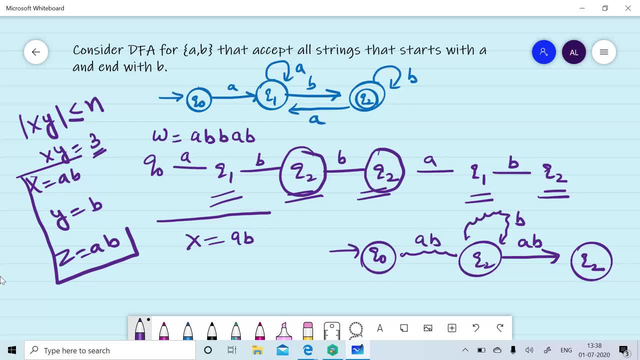 we can able to consider that x as a b, y as b and z as a b. so, depending upon the string, we can able to decide x, y and z and we can able to divide the string w into three parts, with the condition that the length of y must be greater than 0 and the length of x? y is less than equal to n. 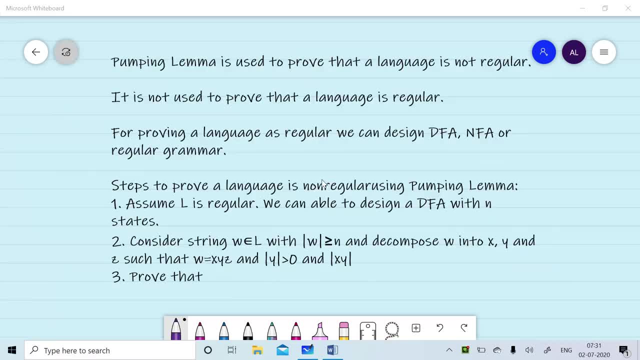 where n is the number of states. pumping lemma is used to prove that a language is not regular. it is not used to prove that a language is regular. if we want to prove a language as regular, we will design dfa, nfa or regular grammar for the given. 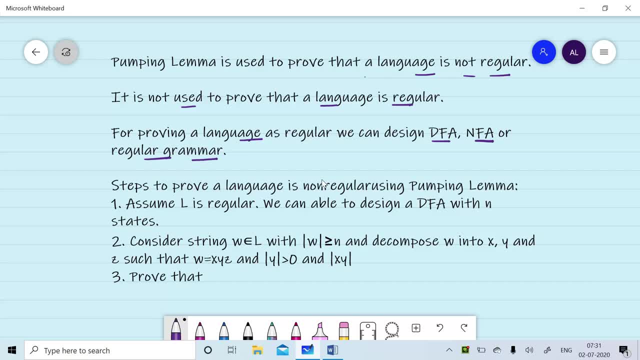 language. following are the steps used to prove a language as non-regular using pumping lemma. in the first step we will assume the given language, l, is regular. so if the given language is regular, we can able to design a dfa with n states. in the second step, we will consider string w. 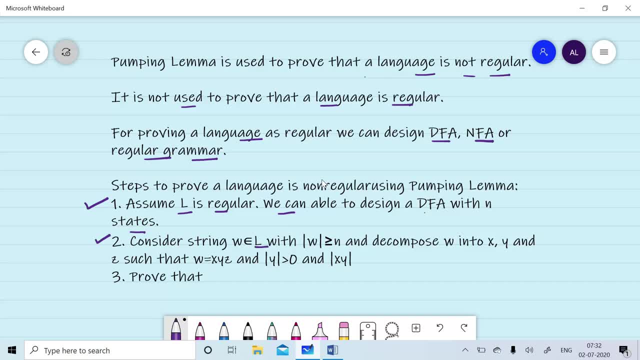 belongs to the l, such that length of w is greater than equal to n, and we will divide w into x y z, such that w is equal to x y z and length of y is greater than equal to 0 and length of x? y is less than equal to n. 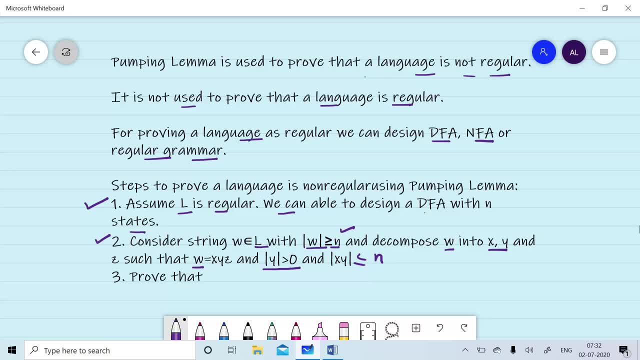 in the third step we can design a dfa with n states. here, for example, we want to design the string: w is less than equal to z and x, y is less than equal to n. third step: we will prove that x, y, i, z does not belongs to L, So we will prove that a. 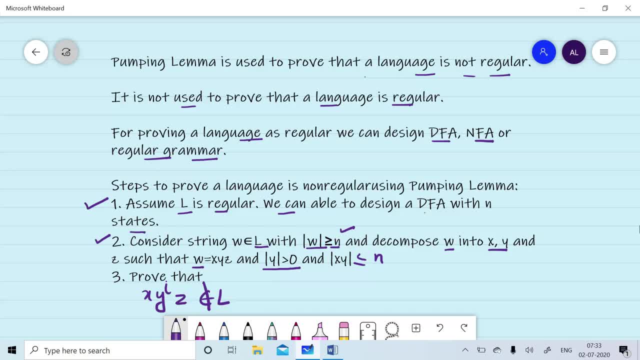 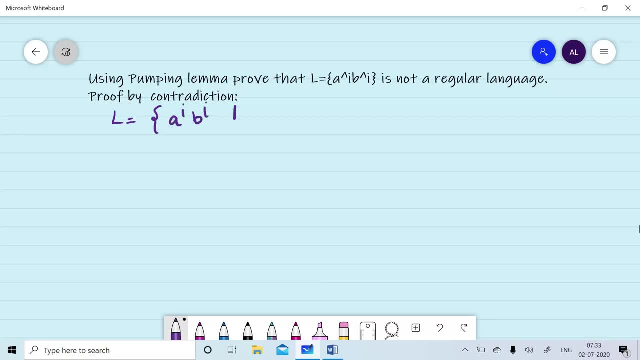 language is non-regular using the proof of contradiction, Suppose, given the language L, a, i, b, i, where i is greater than equal to 1, and we want to prove that this language is not a regular one. So in the first step we will assume L is regular, so there exists. 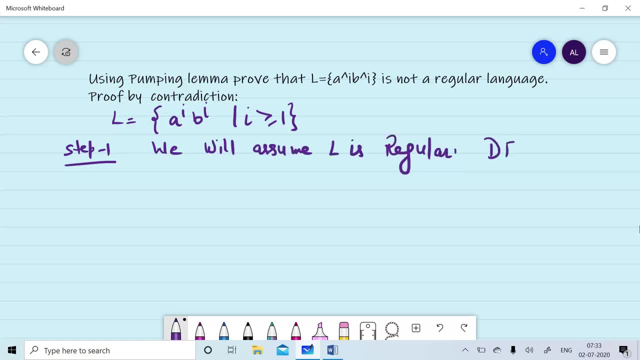 a DFK with n states In step 2. let's consider W such that 2M is greater than equal to n. Now we will divide – W equals to 2m appearing in middle page, and there is also a good chance that N will be. 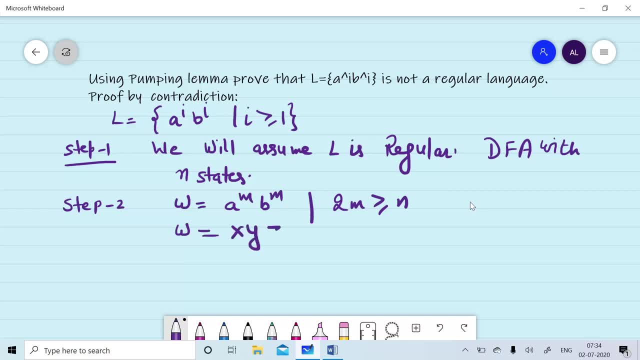 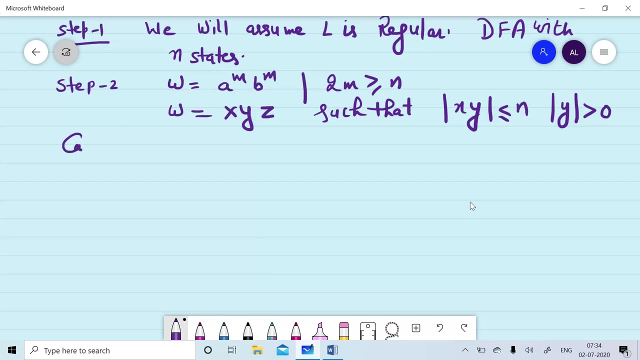 to three part, x, y and z, such that length of x, y is less than equal to n and length of y must be greater than zero. So following cases can occur: case number one: in case number one, y can be of the form a raise to power, k. case two, y can consist of a number. 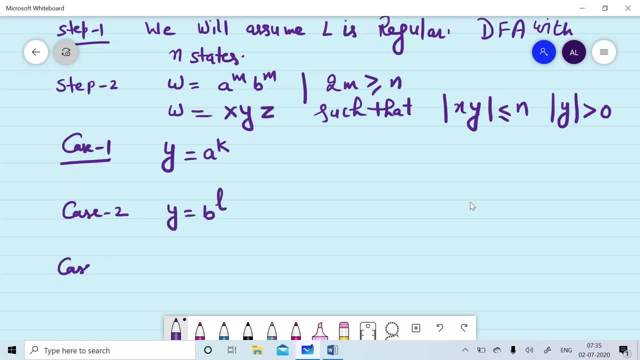 of b, case three, y can consist of a number of a and a number of b. Now x, y, z is a, m, b m. consider i equal to zero. so x, z is nothing. it is a m minus k, b m, where k is. 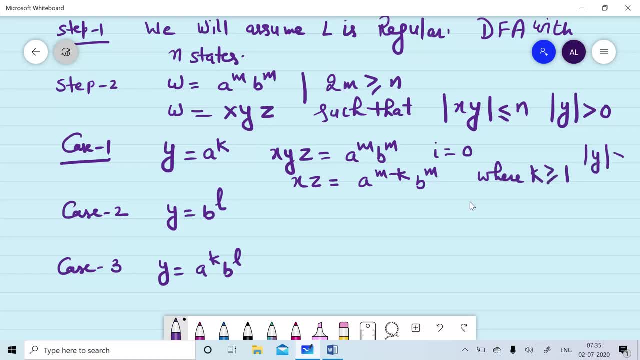 greater than equal to one, because length of y must be greater than zero. So m minus k is not equal to m. so number of a followed by number of b are not equal. x? z does not belong to l. what it means? x, y, power, i z does not belong to l. so if 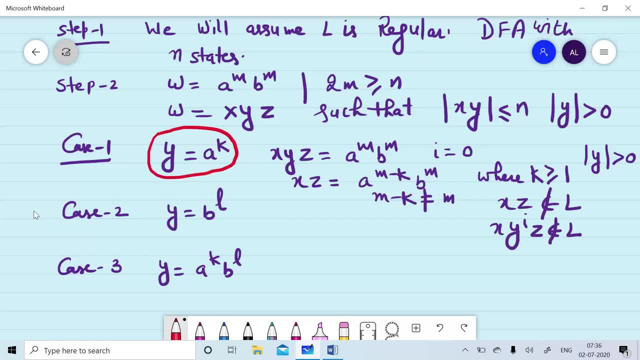 we will consider y equal to a power k, then x- y power i z does not belong to l. similarly, if if y is b power n, it is veryуш, then x- y power i z does not belong to l. similarly, 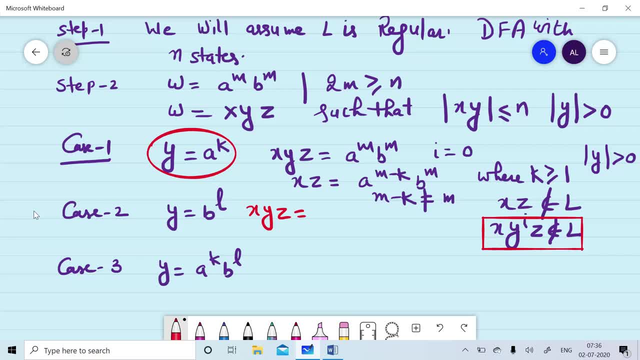 L, then W can be divided into x, y, z, m minus L, For i equal to 0, x, z will remains a, m, b, m minus L, and L will be greater than equal to 1 because the length of y is greater. 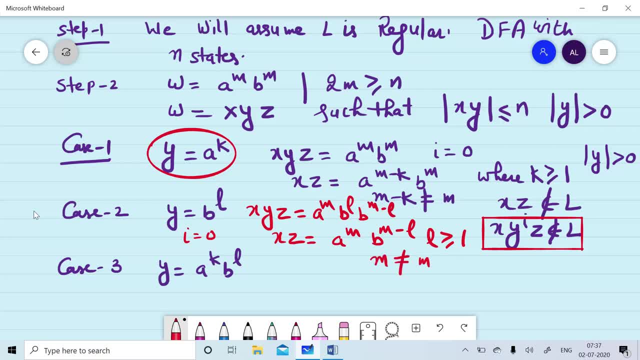 than 0.. m is not equal to m minus L. It means x. z does not belong to L. Now we will consider the third case. Consider: y is consisting of a number of a, followed by a number of b, So